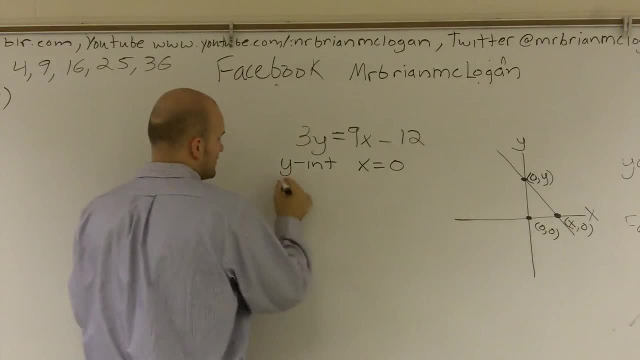 x value is 0, 0. So I know that the x value is 0, 0.. So I know that the x value is 0, 0. And when I'm looking at my x intercept, my y value is equal to 0.. I don't have a y there. 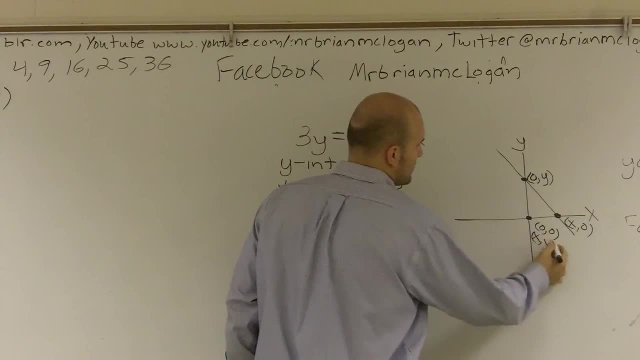 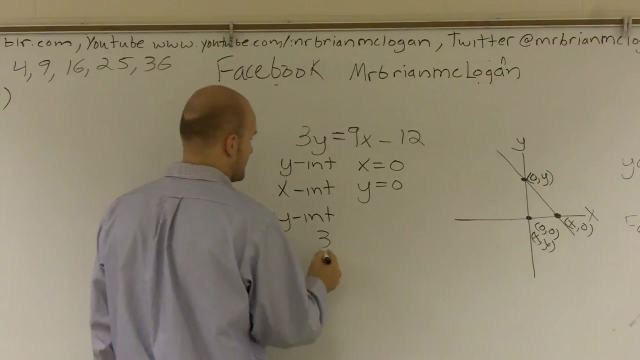 anymore because, remember, all coordinate points are x, y. So if I have a 0 for one of these, I know that that value is 0. So what I'm going to do now is, if I want to find the y intercept, I'm going to plug 0 in for x. So I say 3y equals 9 times 0, and 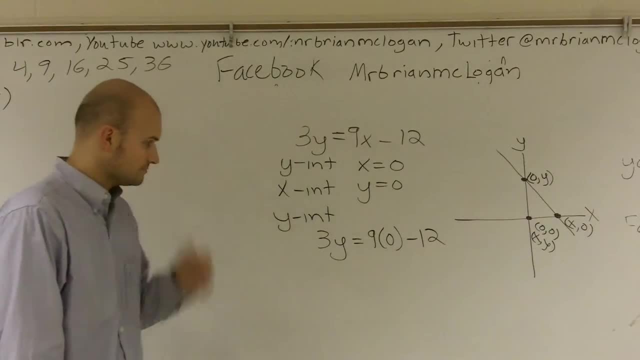 minus 12.. 9 times 0 is 0. So I get 3y equals 0 minus 12.. Obviously I don't need to keep my writing to 0, but I figured I'd be nice to you. I want you to see where everything's. 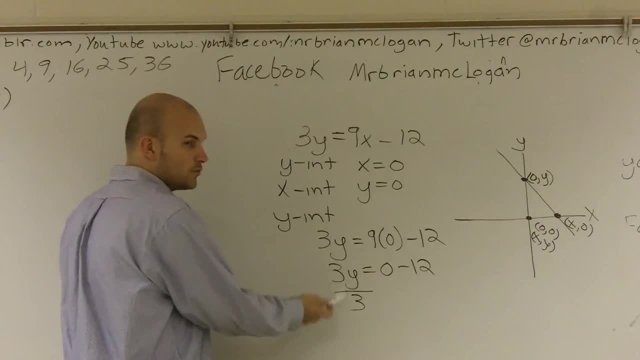 coming at for us. So now I divide my 3s. 3 divided by 3 gives me 1.. 1 times y is y, And I divide 3 on this side And what I obtain is negative. 12 minus 3 is a negative 4.. So 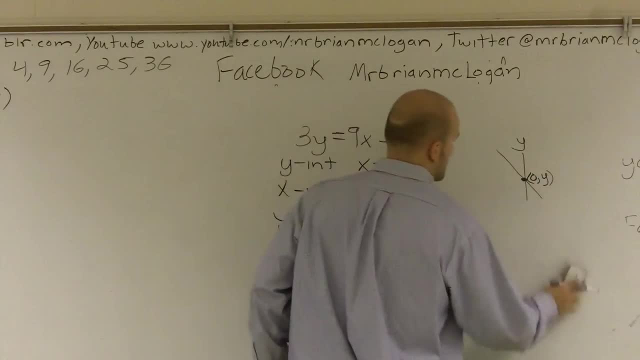 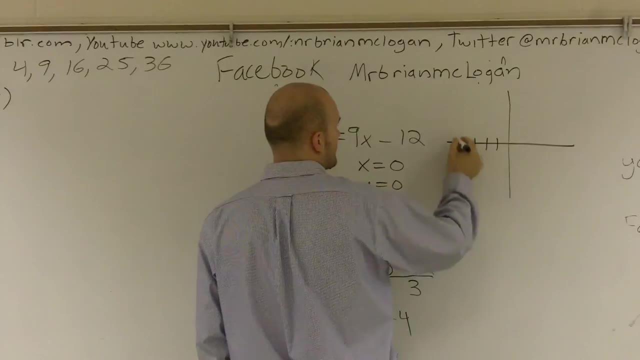 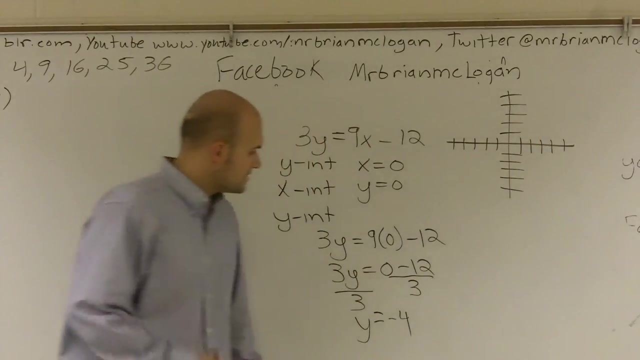 let's actually Let's put some points up here: 1,, 2,, 3, 4, 5.. 1,, 2,, 3, 4, 5.. All right, So if I know my, y equals negative 5 when x equals 0.. x equals 0, y equals negative 4.. So x equals. 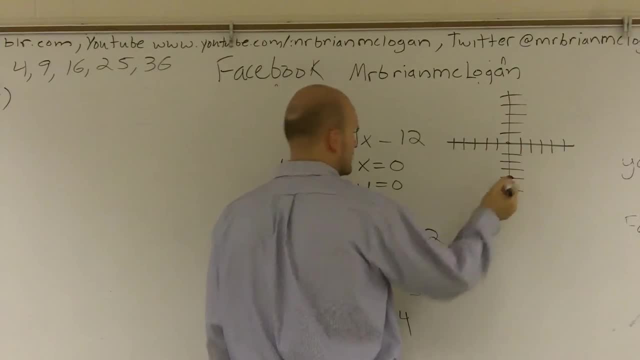 0, y equals negative 4.. 1, 2, 3, 4.. 1, 2, 3, 4.. 1, 2, 3, 4.. Next point: x-intercept: y equals 0.. 3 times 0 equals 9x minus 12.. 3 times 0, obviously. 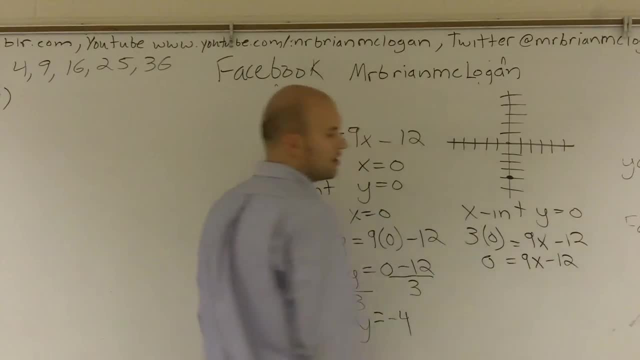 is 0 minus 12.. Now I need to solve for my x. right, I need to get everything off the side of the x. So to do that, I need to say what is happening to my variable. I need to add the 12.. 12 equals 9x.